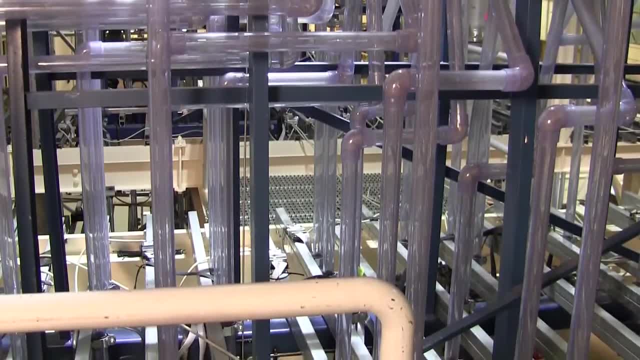 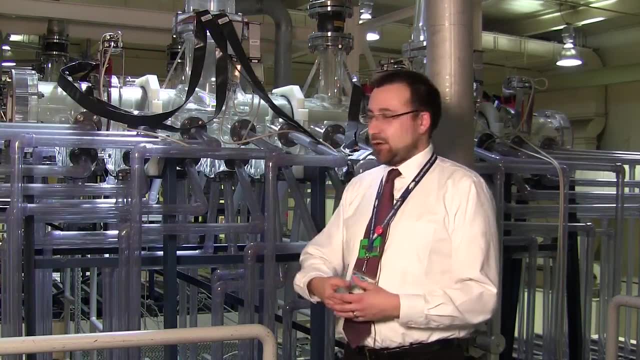 scenario of an accident, the reactor can continue to cool down the fuel bundles and shut down safely. In a reactor you have very high pressures and fairly high temperatures as well, And under accident scenarios that we're interested in, like a loss of coolant accident, 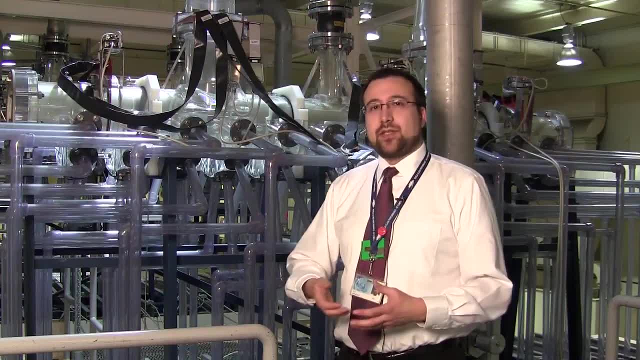 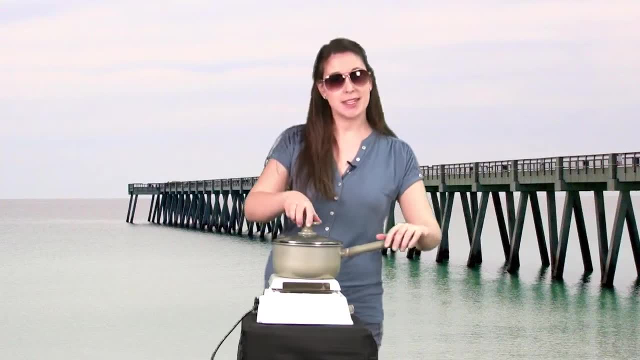 you'd have a break in a pipe somewhere and that would lead to the system depressurizing. Temperature and pressure are two properties of fluids that are related to each other. For example, this pot of water boils at 100 degrees Celsius here at sea level. 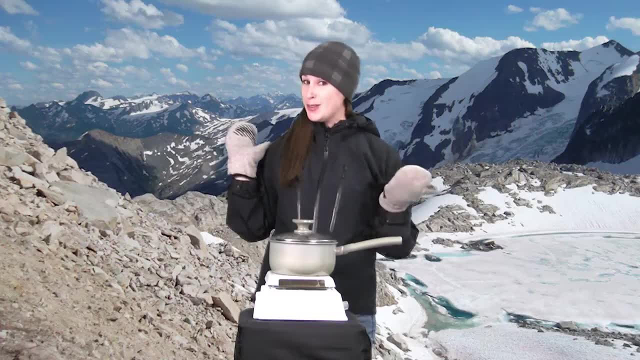 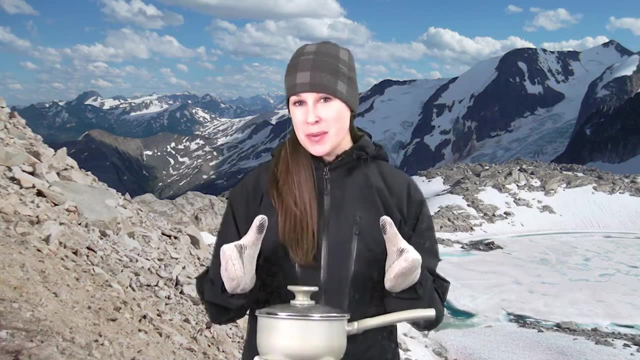 But if I move my pot of water up to the top of a mountain at about 6,000 meters, the water would actually boil at a lower temperature about 80 degrees Celsius. That's because the air pressure up here in the mountains is actually lower than at sea. 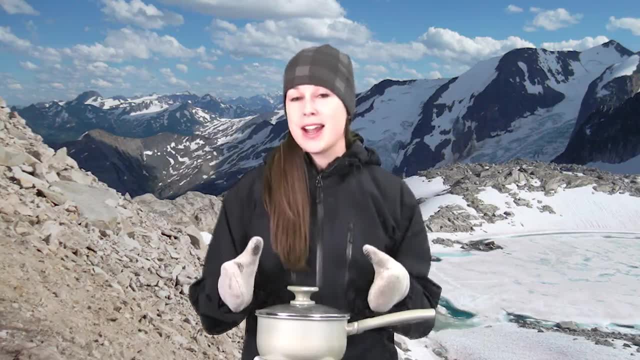 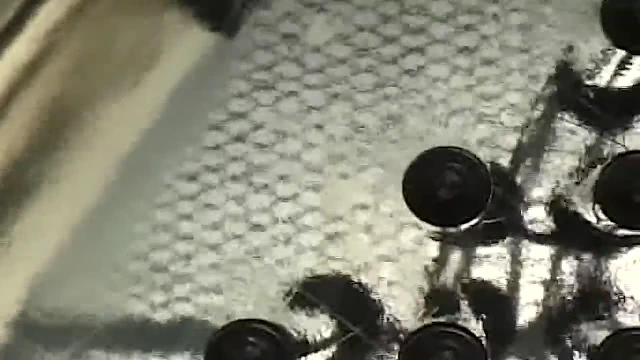 level. The boiling temperature of this water is about 80 degrees Celsius. This water decreases when the air pressure decreases and it takes less heat to boil this water. The water coolant inside the pipes is a lot like the water in the pot, sitting at a comfortable. 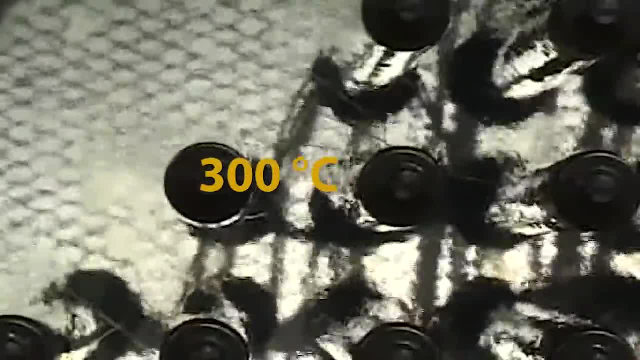 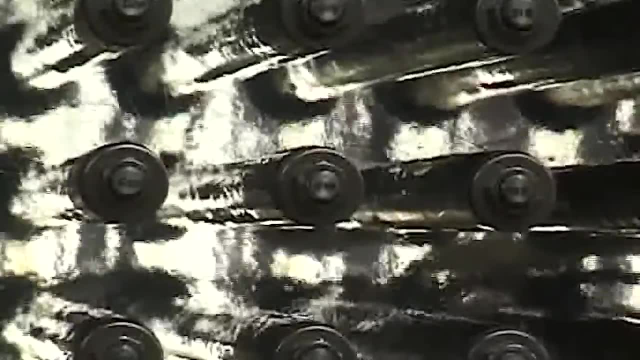 300 degrees Celsius, but still not boiling, because it's at 100 times the normal atmospheric pressure at sea level. If a pipe breaks, however, the pressure will decrease and the water may start boiling. Steam would start forming and boiling. We're interested to see. where does that air go? 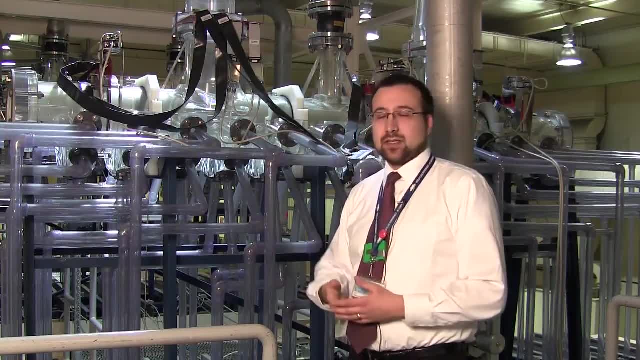 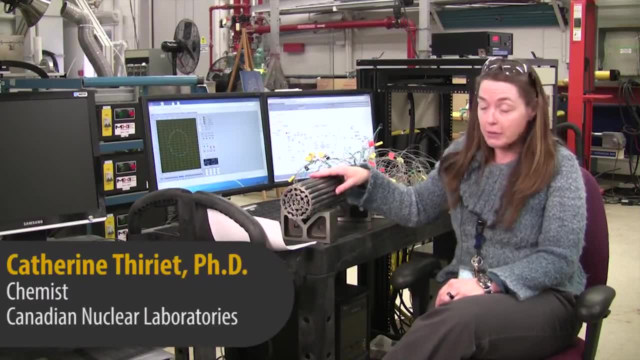 If you get certain channels that fill with air, that could be an issue Because of course that would mean that there's less heat transferred from the fuel to the coolant. When the temperature increase of the bundle, the bundle itself will deform and inside. 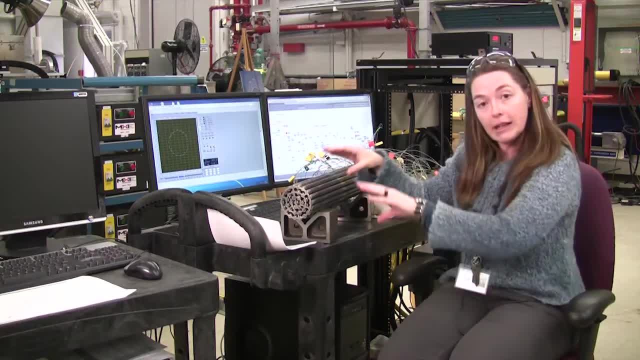 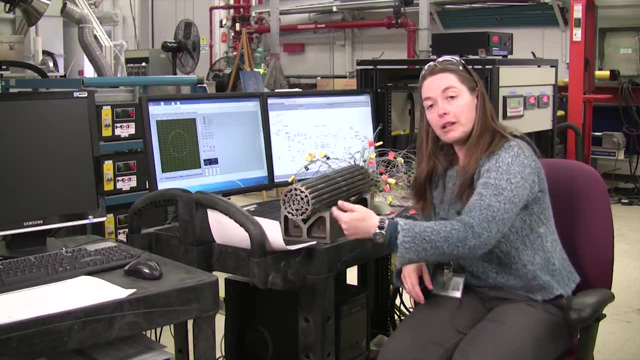 you see, the sub-channel will be closing up. the gap between the fuel element will close up, So it means that the coolant will not be able to pass through and remove the heat. This physical behavior of the fuel bundle is studied using special apparatus in Catherine's. 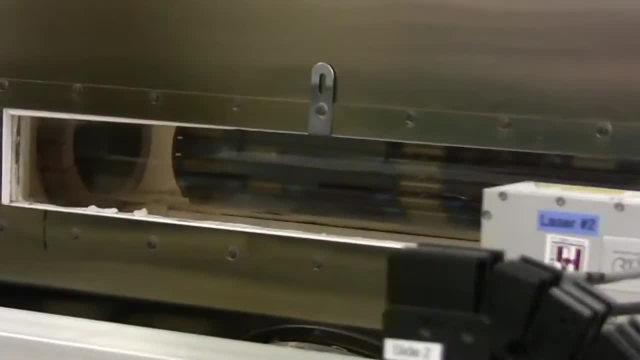 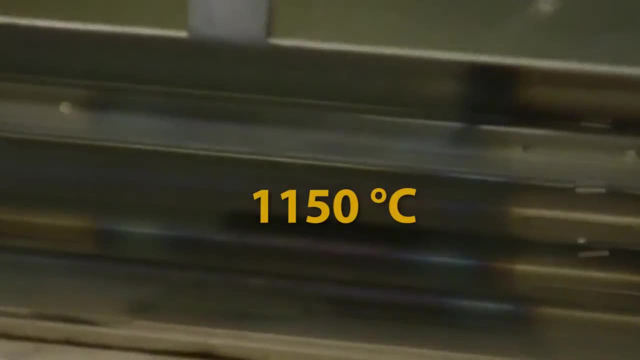 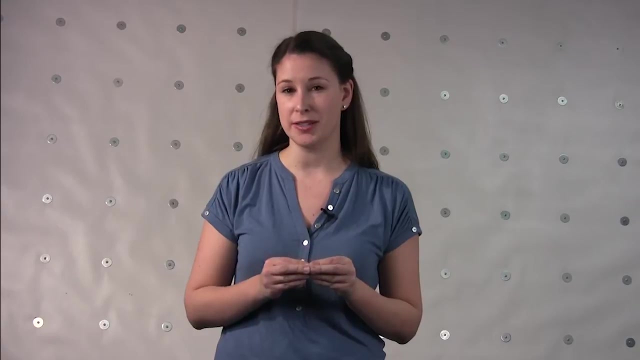 lab. Lasers will scan the bundle back and forth as it's heated up, with super-heated steam coming out at a whopping 1,150 degrees Celsius. Fuel bundles can survive some tough stuff, but the emergency shutdown systems will put an end to rising temperatures in these fuel bundles long before they can reach the temperatures.